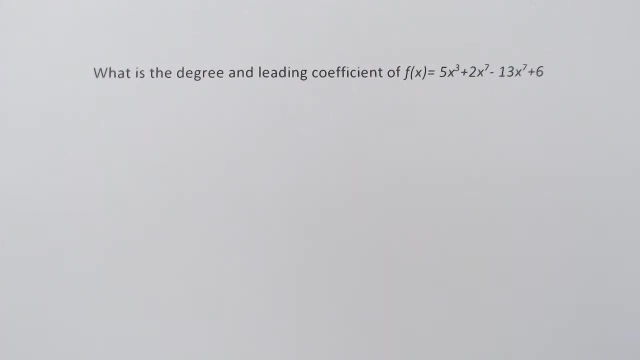 Hello and welcome back to another episode of Math with Sohn. Today we are going to be talking about a midway point between polynomials and going over and reviewing it, So I got several problems printed out that we're going to deal with. The first one is asking about the degree and the 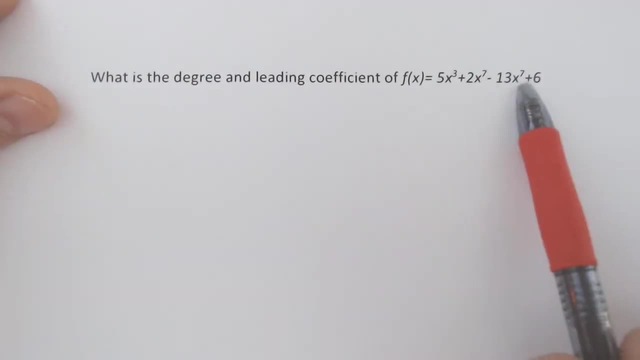 leading coefficient of this. So you have to pay attention to the way that it is presented and also be very careful, because this one is especially different, because the leading coefficient would have been either 2 or 13, but notice how both of those are x to the 7th. Well, if you have 2, x to 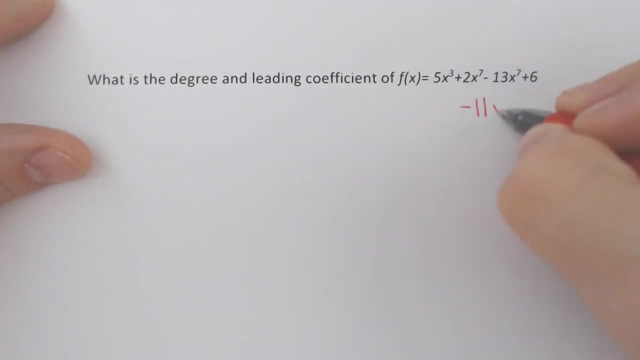 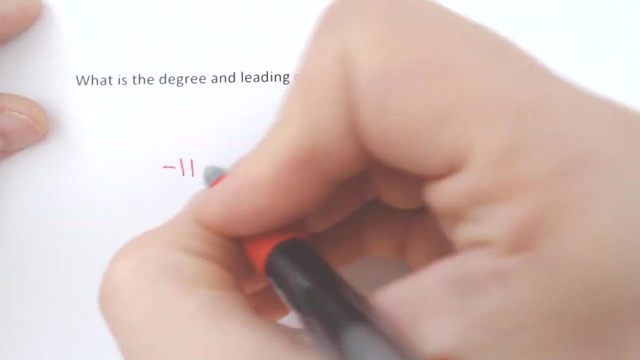 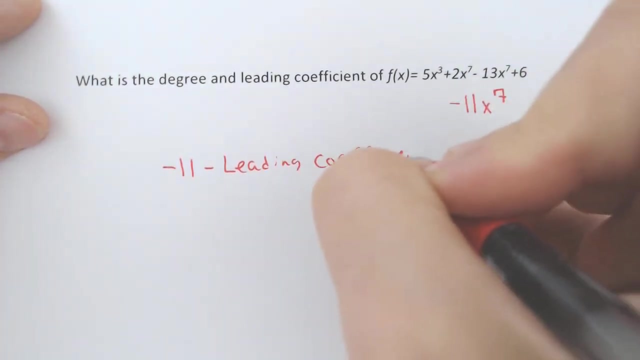 the 7th and negative 13 x to the 7th. they combine to make negative 11 x to the 7th and the 11 is going to be the negative. 11 is going to be the leading coefficient, and, and, and, and the degree is going to be the 7.. So the degree is going to be the 7, because that is the biggest. 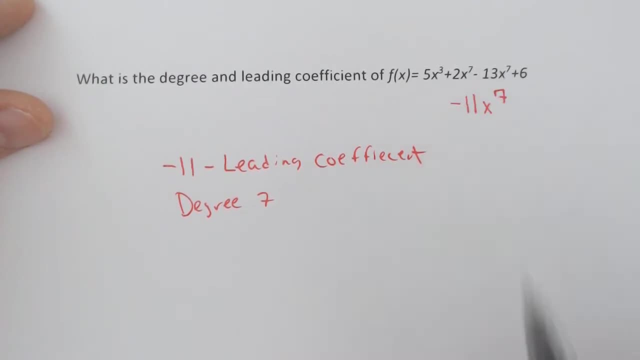 exponent and you just had to be careful because there were 2 x to the 7th, so you had to combine them first. They were trying to trick you, Alright. next one: compare the end behaviors. So when you're comparing the end behaviors then you got to take like what's going on between both of these? So 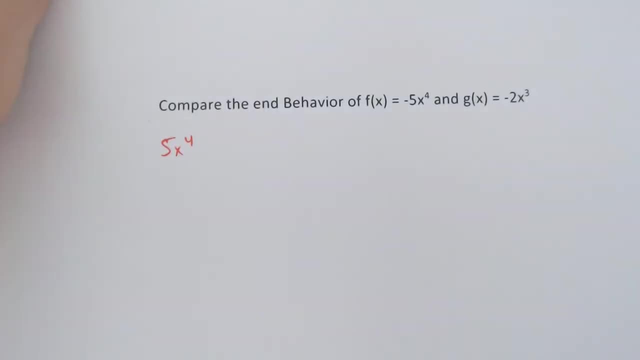 if we take the 5 x to the 4th, the negative 5 x to the 4th, if we graph that, it would look something like this: It would kind of do some squiggles and it would be kind of looking like it's ending in a negative direction on the left and the right. And if we graph the negative, 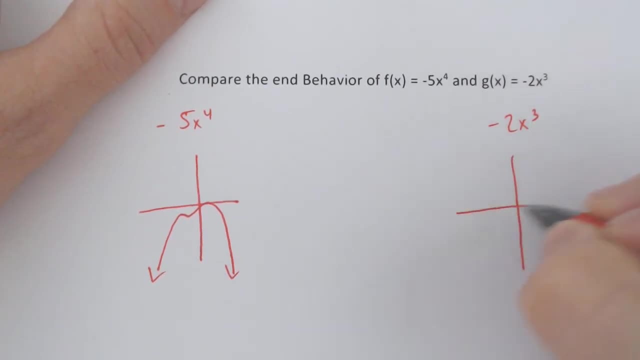 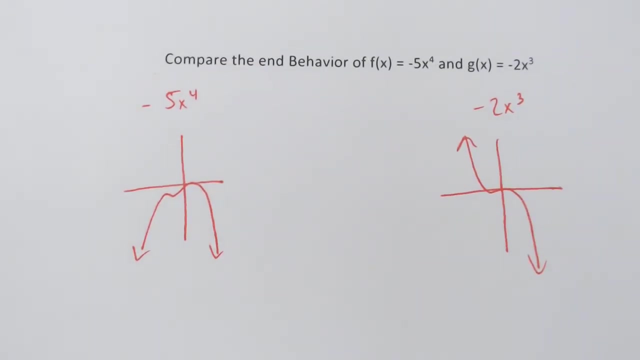 2 x to the 3rd, that one would be going down from left to right with some squiggles in the middle. So the way that you're going to compare, that is, you would say, as x approaches infinity, x approaches infinity. they are doing. 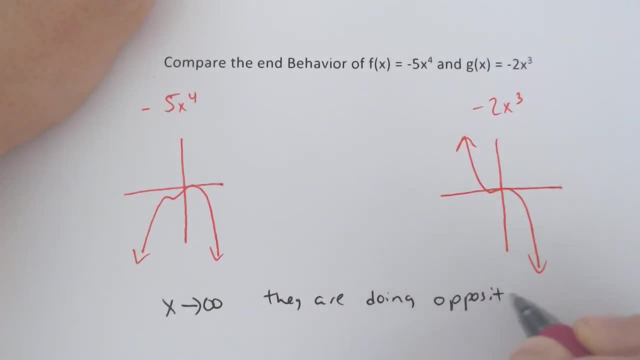 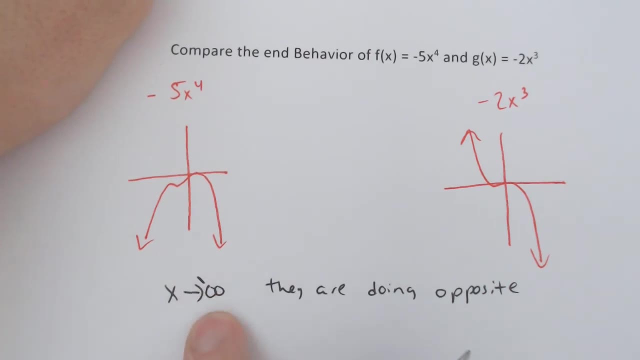 opposite things because, excuse me, negative infinity on the left side, negative infinity. they're doing opposite things because on the left side, we're going down over here but we're going up over there, And this would be the left and this would be the left, and that's what we're talking about here: the left side. 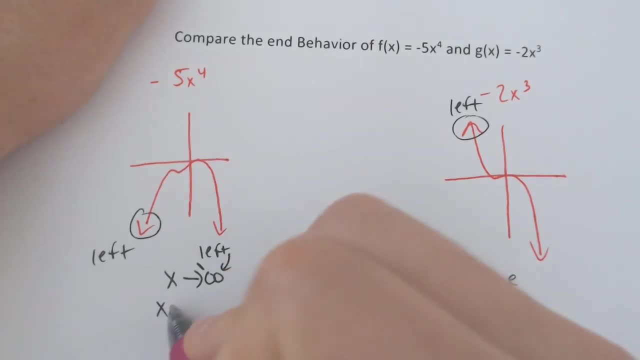 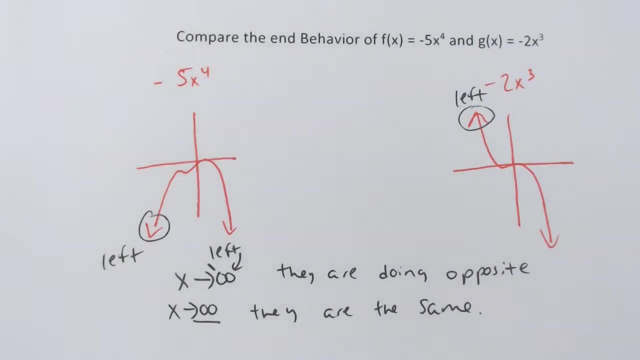 That's the left, But on the left side, the right side. as x approaches positive infinity, they are both going down. so, as we are going to the right side, they are the same, and that would be how it would be worded and how you would need. 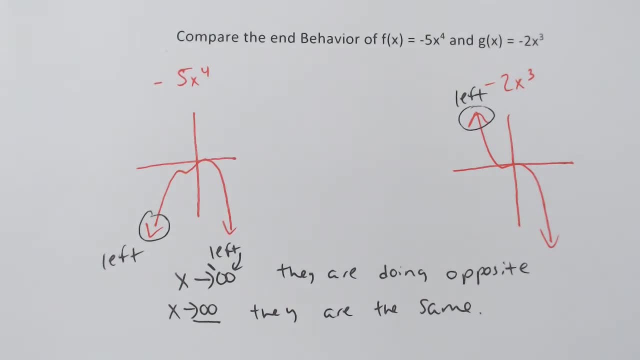 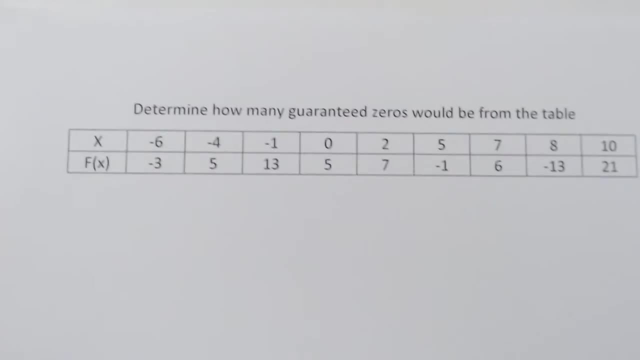 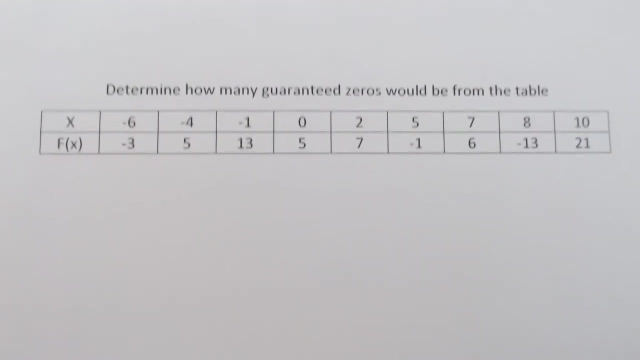 to understand it for some things. you could also just write the entire end behavior if you wanted to. all right, next up on the table. no pun intended, we have a table. okay, when you're determining what is going on with this table, then you need to look at it and you have two choices. you can plot every. 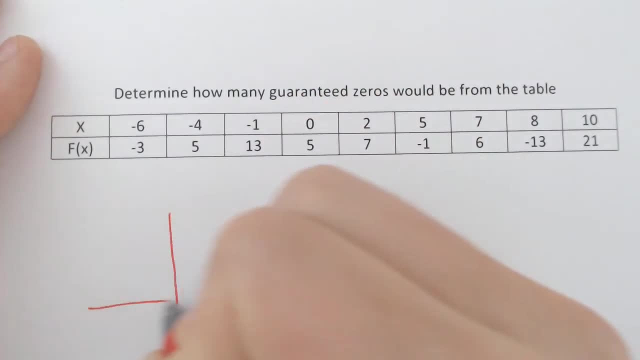 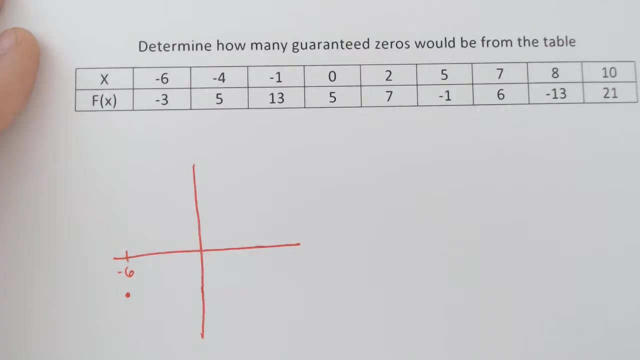 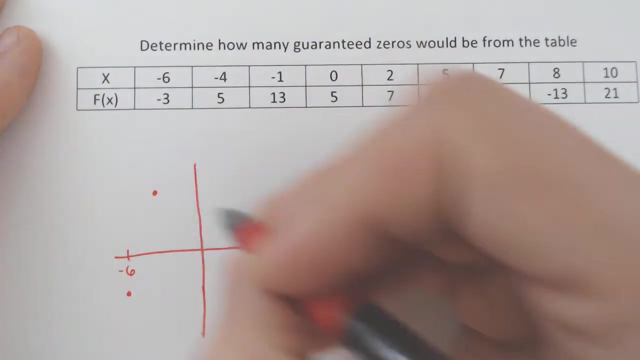 single one of these points real quickly. and when you plot every single one of these points, you would plot negative six, negative three dot. you don't have to be perfect. and then negative four, positive five up here, negative 113, a little higher if we started connecting them. 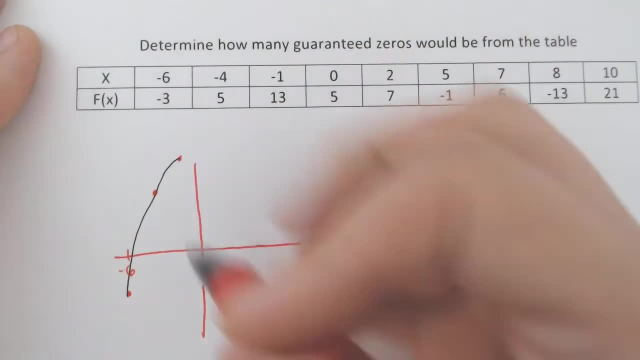 the dots, we would end up with something like this: at zero we start going down, we're at five, so it'd start going down, and then at two we're back up at seven, which tells me that it changed direction, which maybe there was a zero, but we don't know. for 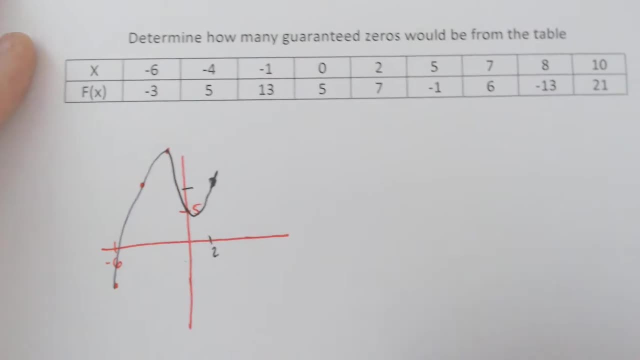 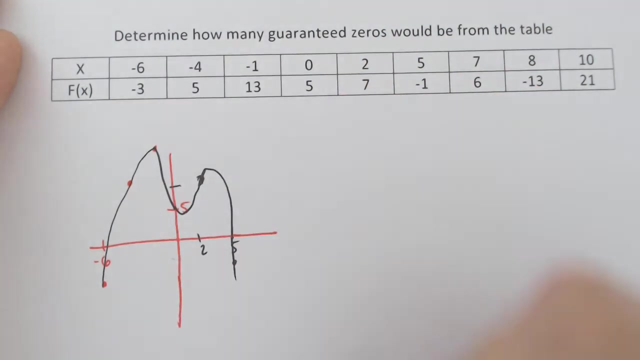 sure, maybe it only dipped down to right here, and then we could plot the point at five and we'd be at negative one, so it'd be down here, and then we'd be at negative one, so it'd be down here. it went downward and then at two, at seven, we're back up at six, way up here. so it's going back up. 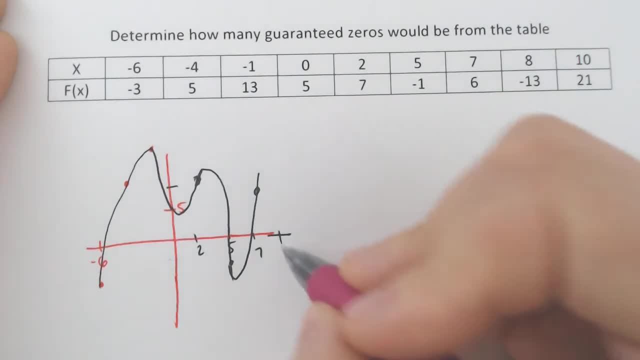 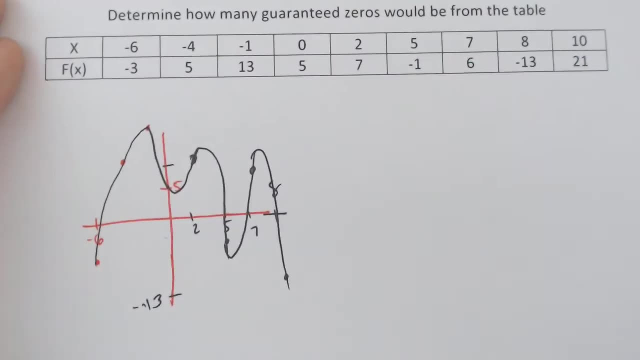 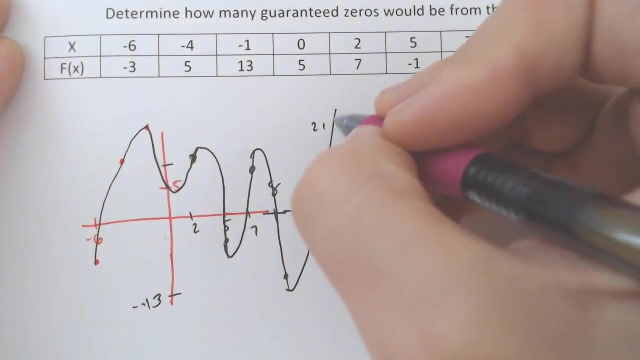 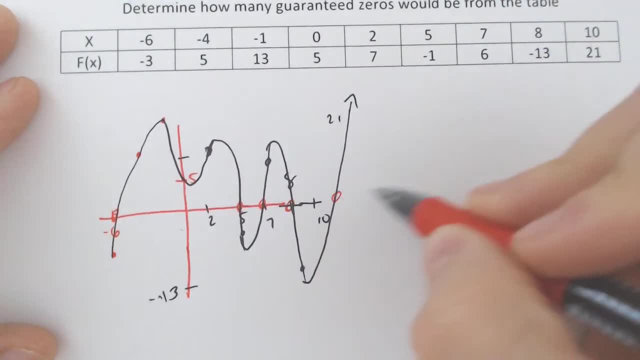 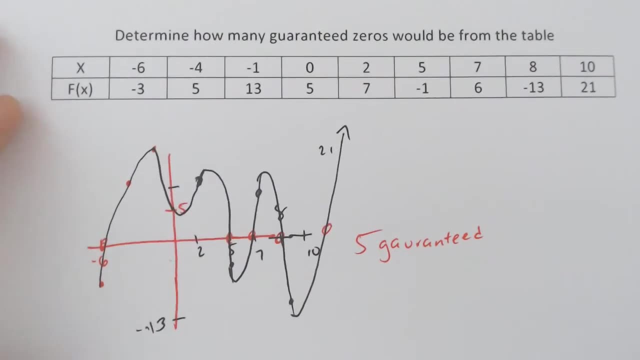 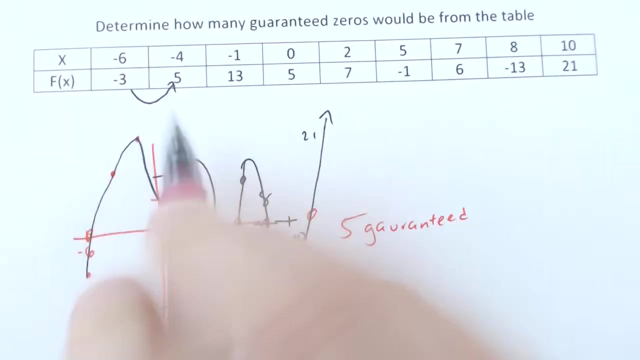 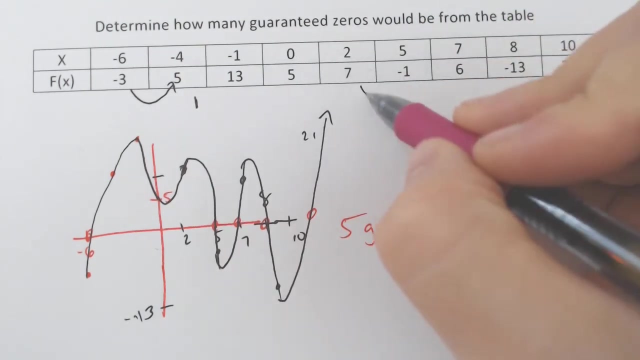 two, three, four, five guaranteed zeros. now, an easier way to do it is to quite literally just look and say: all right, how many times do we change from positive to negative? and this would be one time, from here to here, from negative three to five, that would be one. and then we did another change, from seven to negative one. 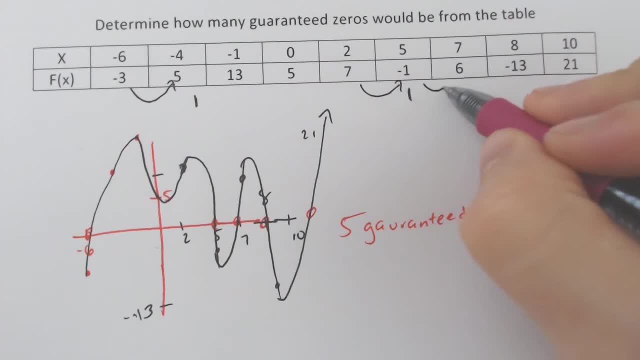 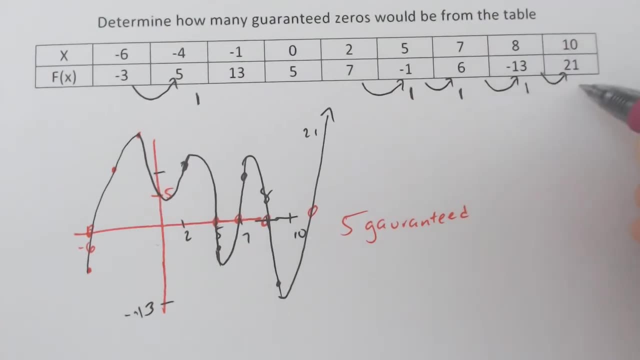 that'd be another, and then another change from negative one to six. that'd be another, And then another change from there to negative 13,. that'd be another, And then another. another change from negative 13 to 21,. which is why 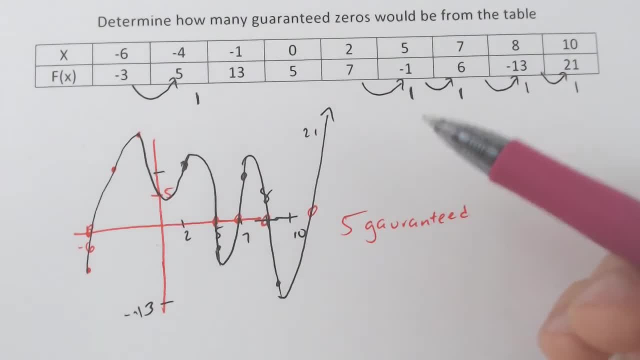 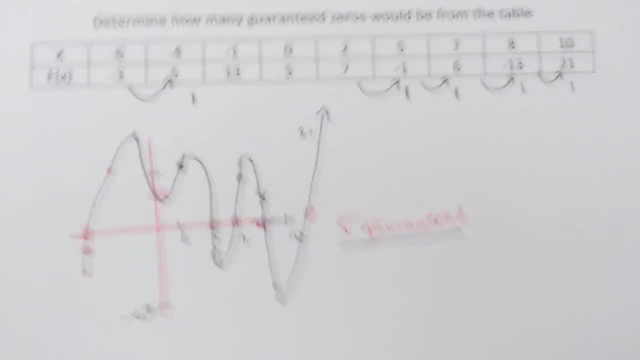 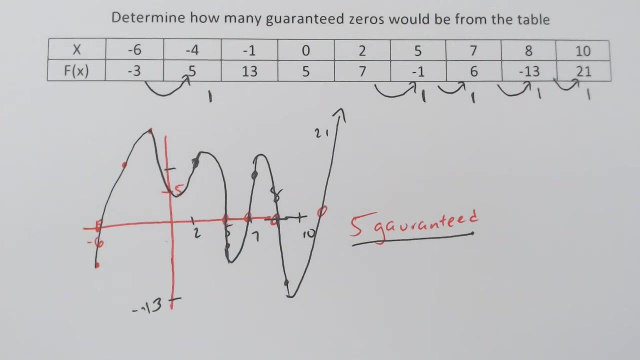 it kind of there at the end, because we had a lot of sign changes And then you could add it up: one, two, three, four, five, five guaranteed. So however many times it goes from negative to positive and then back to negative and negative to positive, it'd be that many guaranteed zeros. 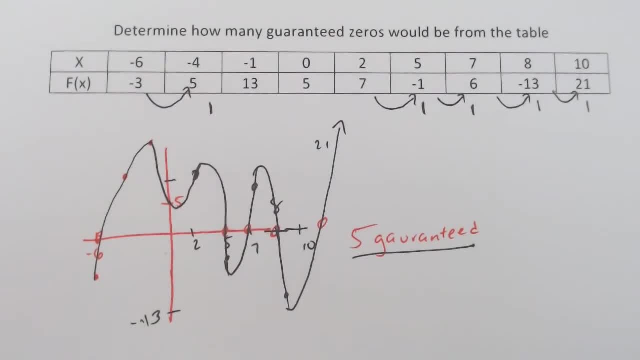 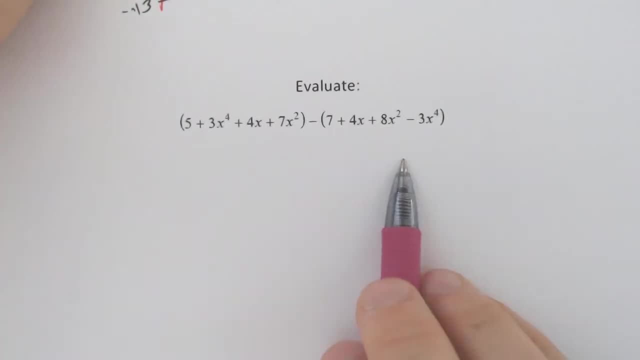 when you're doing it Okay. So that's another method that you could utilize to determine it. All right, Next up, this one's a little easier Evaluate If it's a minus. in between, you need to make sure that you distribute the negative to all of those terms. 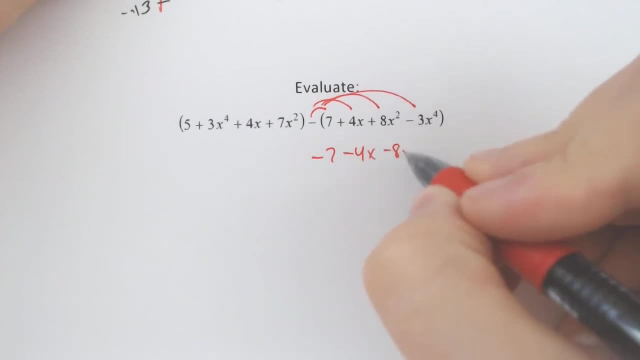 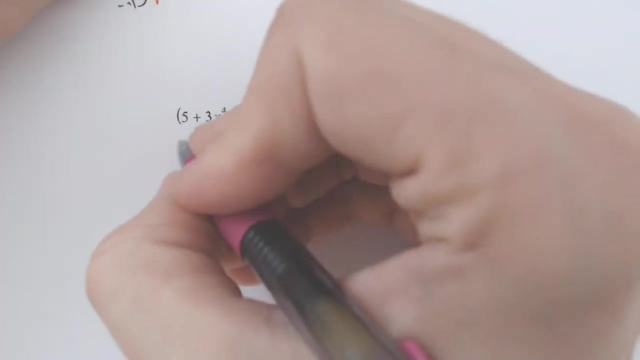 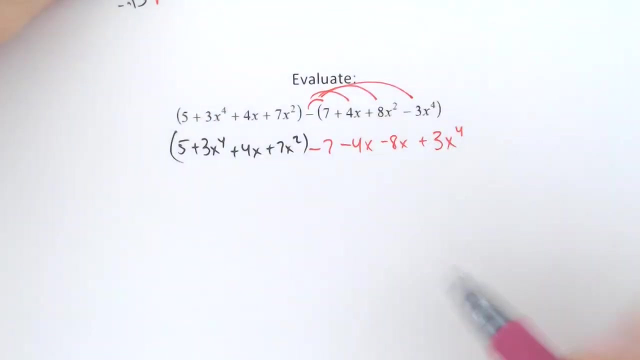 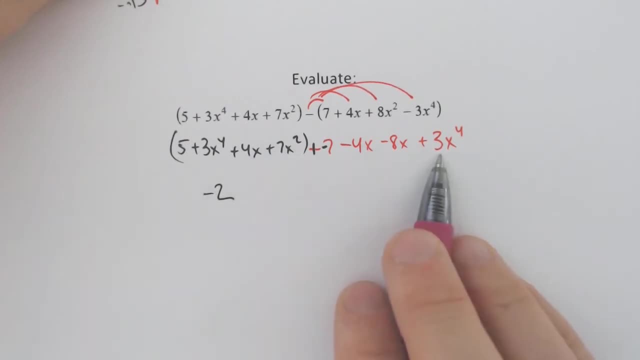 two and three X to the fourth and three X to the fourth makes six X to the fourth, not X to the eighth. You do not add your exponents four X squared, not four X squared, four X and negative four X. They just cancel each other out. 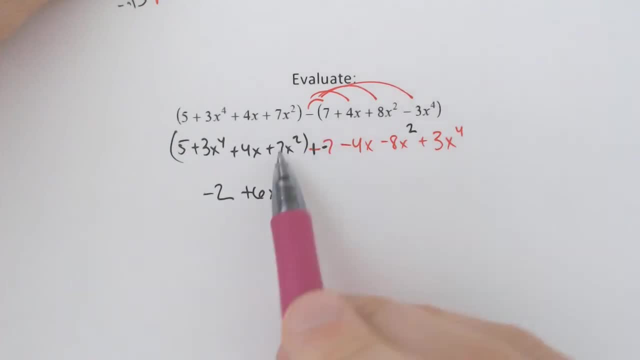 And be careful. I almost forgot my squared here. Seven X squared and negative eight X squared makes negative one X squared. You do not need to write the negative one in front of it, but you can. you're not. you're not, you know, going to be shamed for writing it. 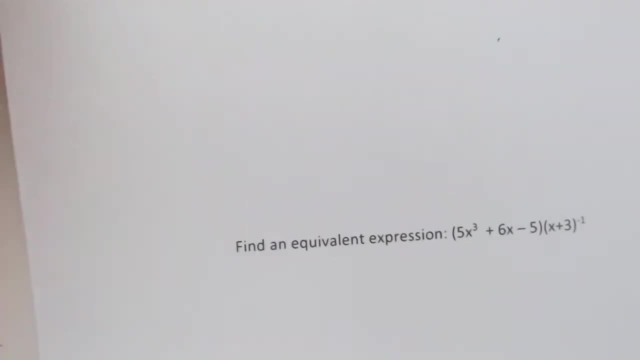 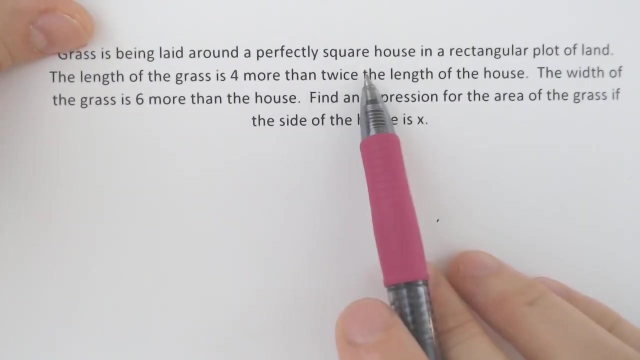 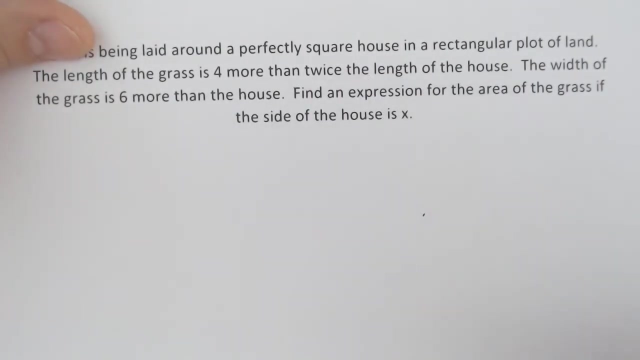 Next page. This next one is perhaps one of the harder ones. You got a grass that's being laid around a perfectly square house And, uh, it's a rectangular plot of land around the with the length of the grass is four more than twice the length of the house. So if we have 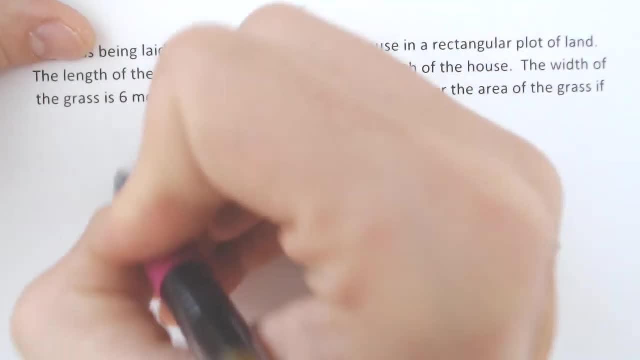 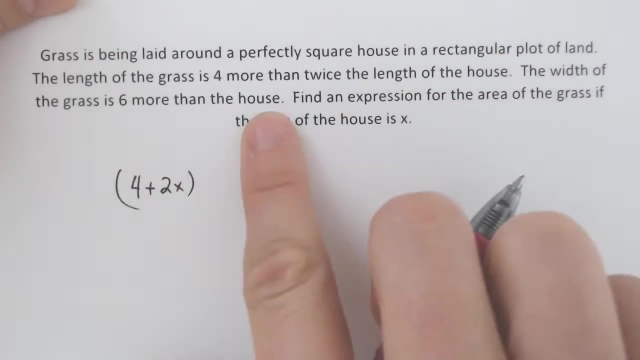 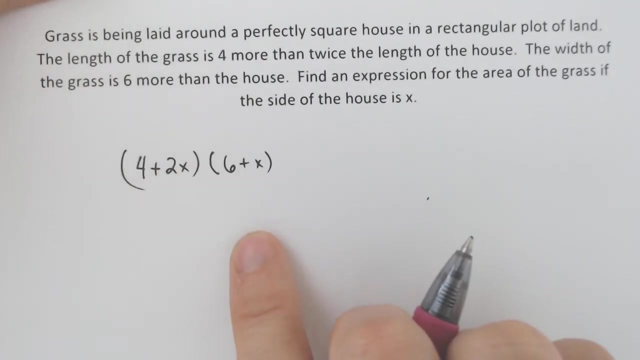 four more than twice of something. that would be four plus two X, So that would represent the length of the grass And the width is six more than the house, So that would be six plus X, or you could write X plus six. All of those represent the same thing And the house side. 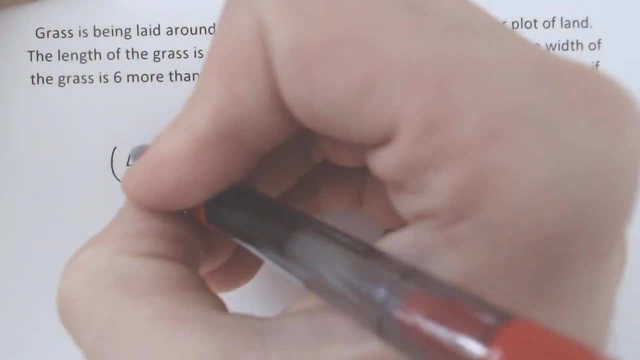 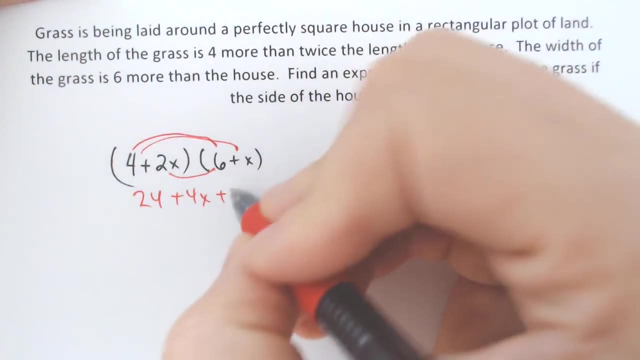 is X. So we're going to foil this out. We're going to have to foil this out. Four times six is 24.. Four times X is four X. two times six is 12 X, and two X times uh, X is two X squared. 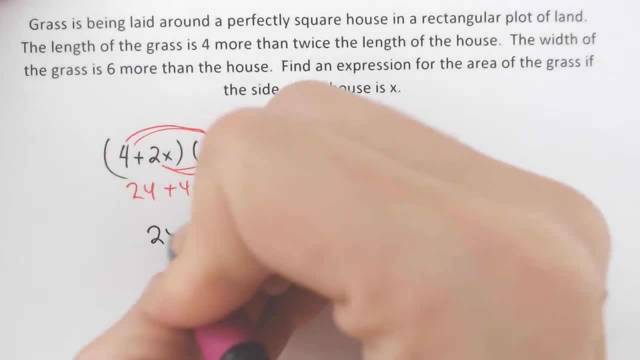 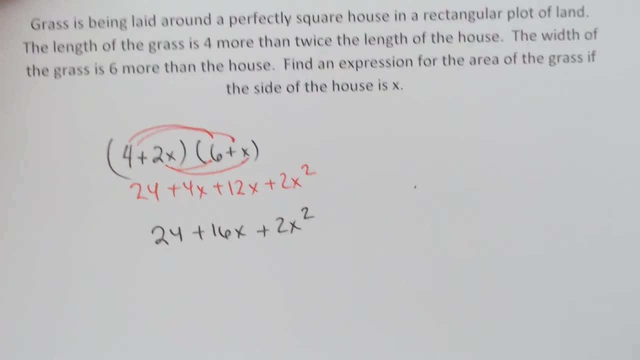 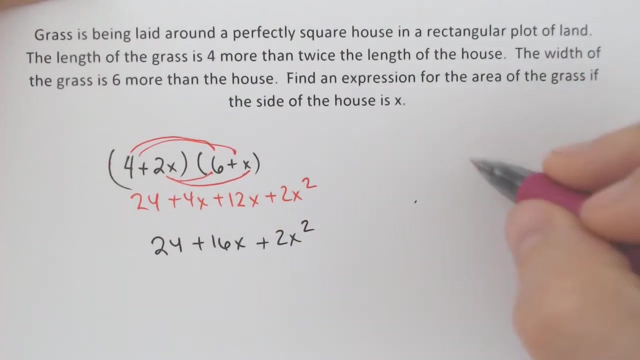 combine any like terms, We got 24 plus 16 X plus two X squared. Now here's the thing that a lot of people forget: We want to find the expression for the area of grass. Um, if the side of the house is X, so we only want the grass. So this is the area of grass. So we only want the grass, So this. 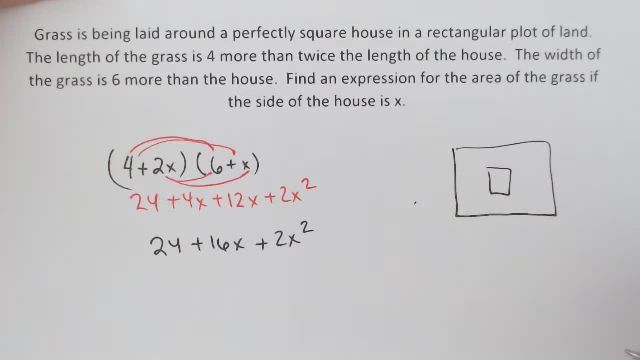 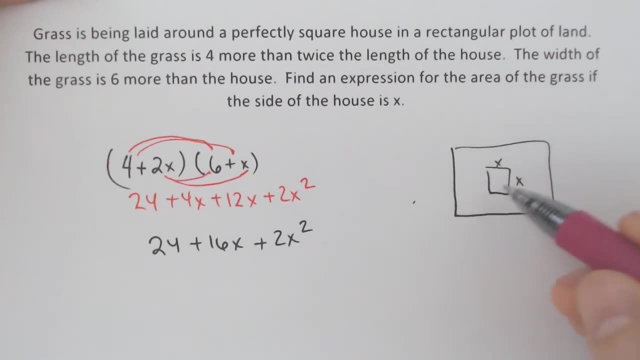 grass is like embedded with a house in the middle, essentially. So what you need to do is you need to. also, if we only want the grass, we have to take this house out. So, if you have to take this house, we've already found, essentially, the area of the house or, excuse me, the entire plot of land with. 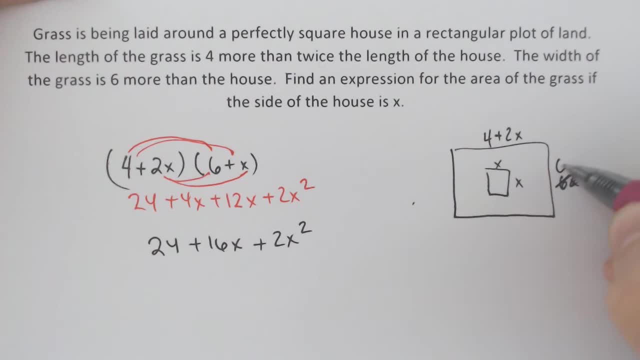 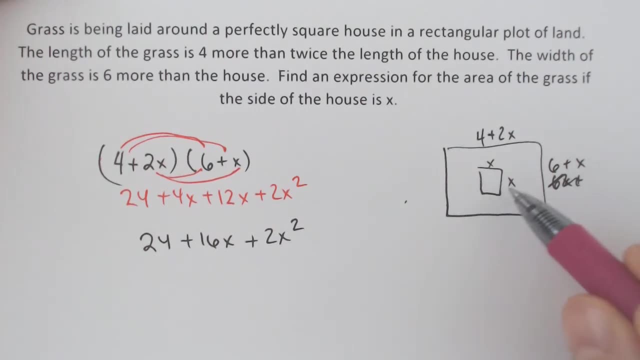 the four plus two X and the six plus six plus X. That's difficult for me to say six plus X. You got to take the the the house away, which the house is just X times X. So you would subtract the X times X, the X squared, which, if you do that, you get 24 plus 16 X. 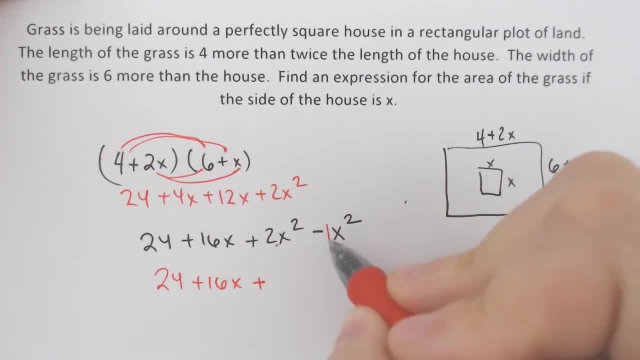 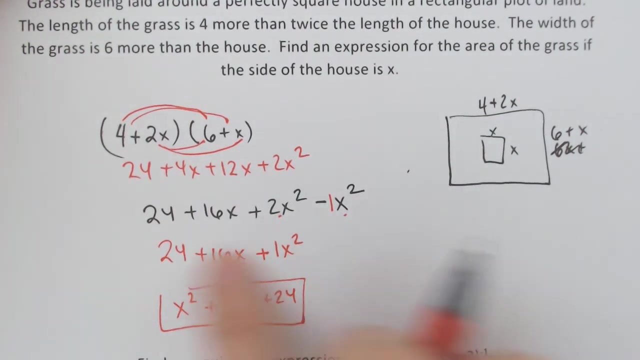 plus two X squared minus one X squared is one X squared, And in most cases you would also have somebody appreciate if you were to write it as X squared, then the 16 X, then the 24,, rather than just the reverse order. Next one on the list. 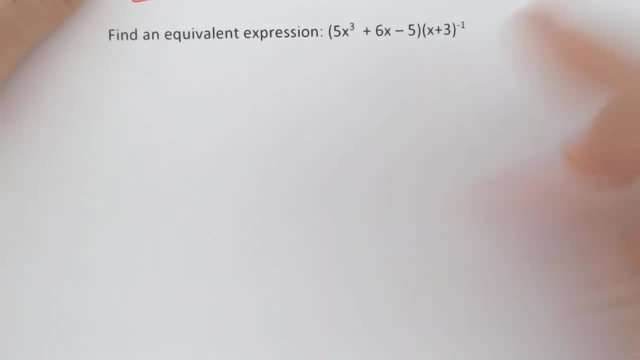 We got find an equivalent expression for this, If you ever see X plus three to the negative one power, anything to the negative one power, and it's only to the negative one power. Typically, that either means inverse, which isn't this chapter at all, or divide, And if it's dividing, 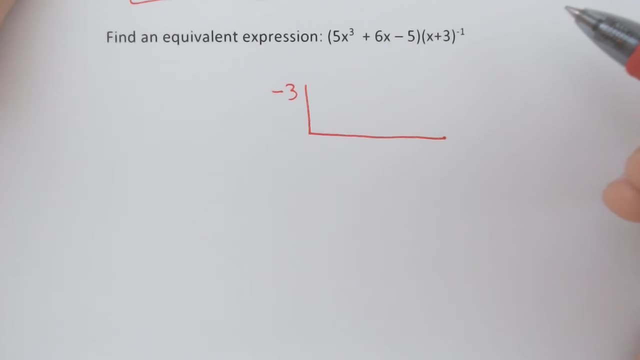 by the basic boring factor, which one of my students is calling, uh, the B, B, F basic boring factor. you would change the sign of the negative three And then you would put these numbers- the five, the six and the five- here. But if you're missing any terms, you gotta put a zero, and we are missing. 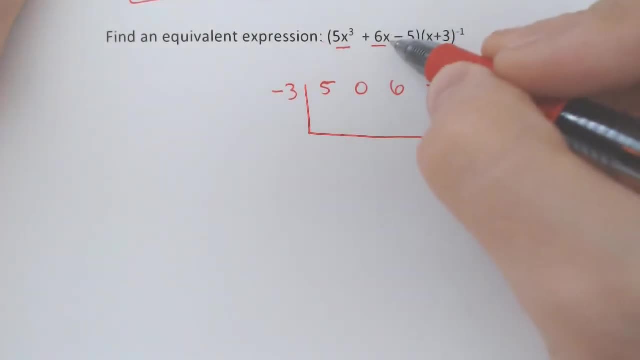 an X squared term. It goes straight from X to the third X. So you need a zero X squared. So that's why I have a zero here. Yeah, Bring down the first number, five. Yeah, Multiply three and five. You get negative 15.. Yeah, Add zero: negative 15 makes negative 15.. Yeah, Multiply three and negative 15,. 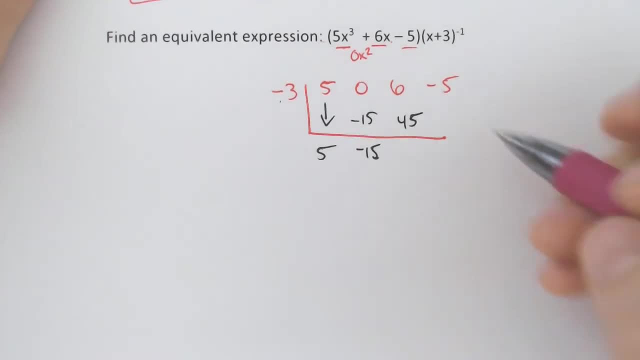 the negative three and the negative 15. You get 45, 45, and six makes 51.. Multiply negative three and 51. You get negative 153. Add straight down negative five and negative 153 makes negative 158.. Whatever you start with, if I started with, 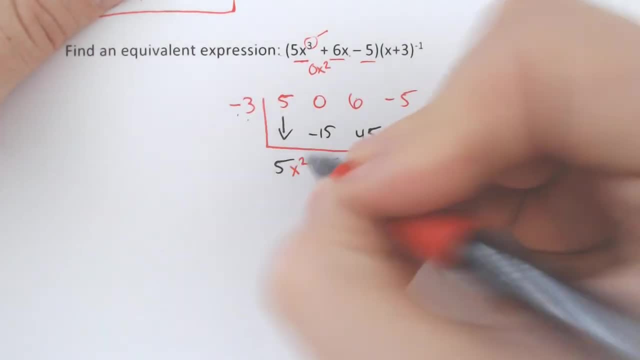 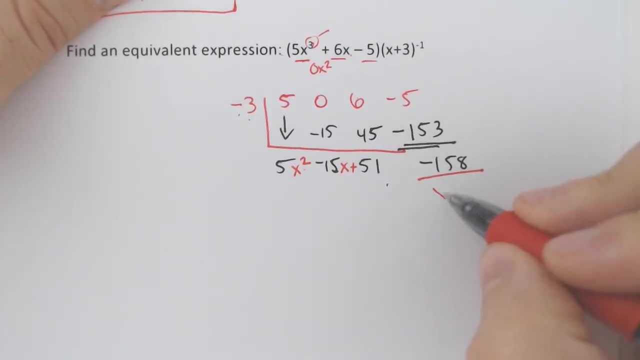 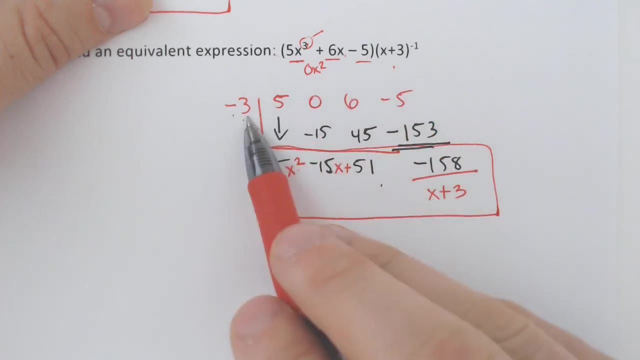 15. Then your remainder, which is the last number divided by the original X plus three. The big thing that you got to remember is change the sign of the three to negative three and make sure you drop the exponent from X to the third down to X squared. 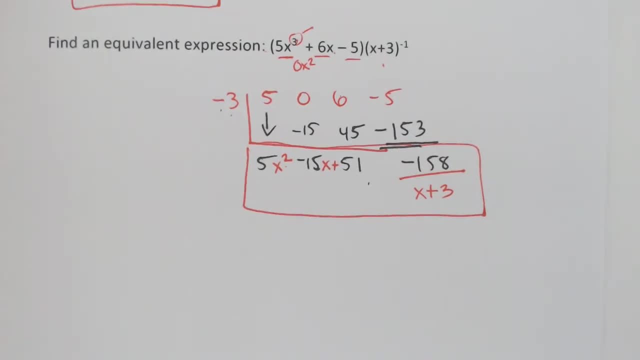 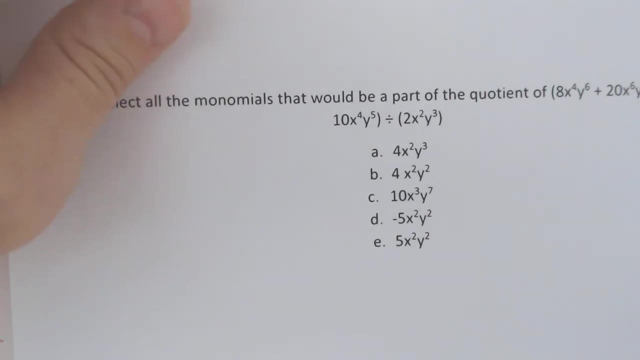 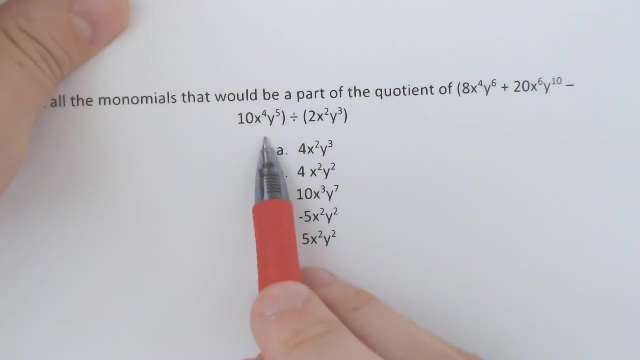 as well as any missing terms you may have. getting right along, We're moving right along. Ladies and gentlemen, we got a few more to go though. A few more to go. Oh, this one didn't print very nicely If we divide this stuff, which goes back over to here, by the two X squared Y to the third. 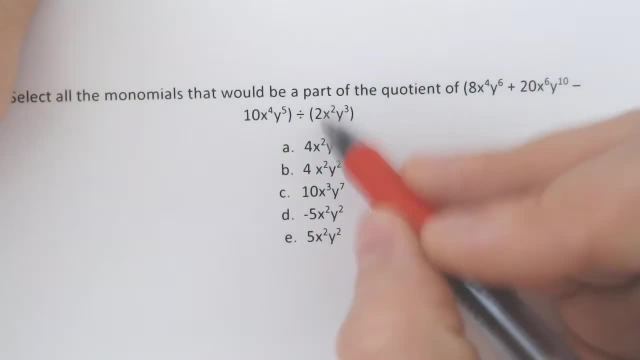 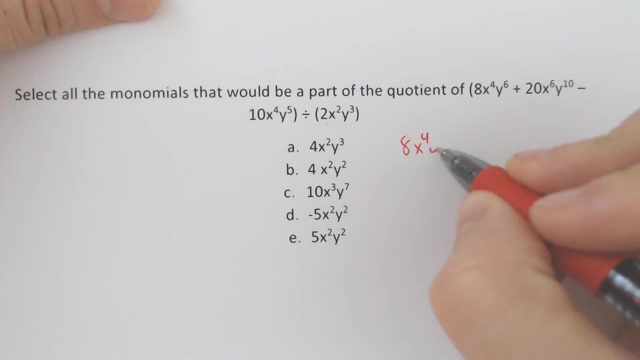 this is not going to be synthetic division, because you're dividing by a monomial and it even has kind of monomial here. You would need to divide everything: eight X to the fourth, Y to the six, everything individually. get their own two X squared, Y to the third, Then the 20 X to the. 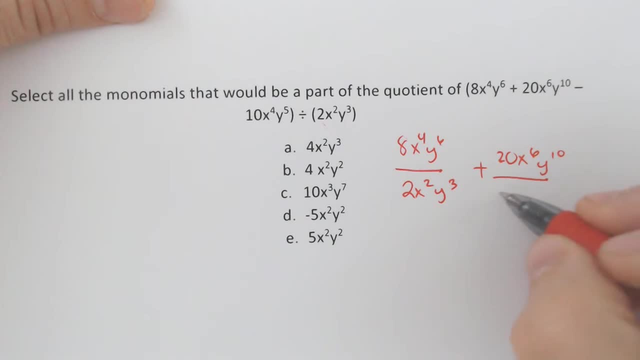 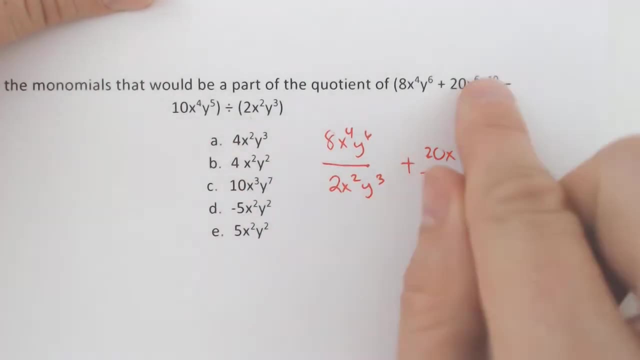 sixth, Y to the 10th, over its own, two X squared Y to the third. Then the last part, the 10 X to the fourth, Y to the fifth, which kind of printed down here: the 10 X to the fourth, Y to the fifth, over its very own, two X squared Y to the third. 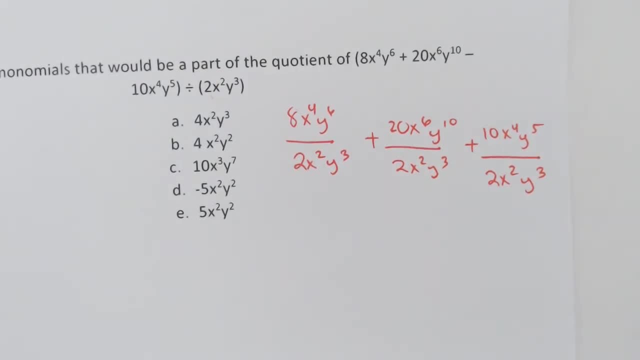 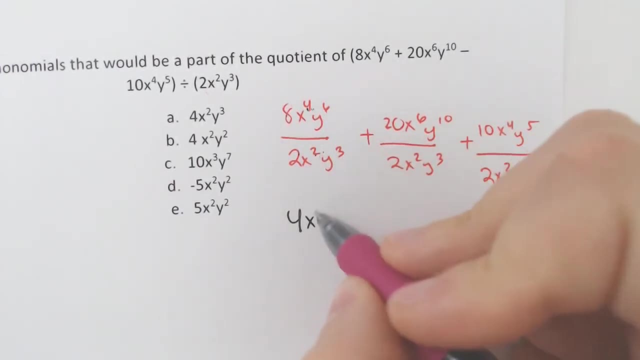 So everybody gets a two X squared and a Y to the third. You divide individually. Eight divided by two is four. Subtract your exponents: Four, take away two, you get two. Six take away three, you get three. 20 divided by two is 10.. X to the sixth. take away two, you get X to the fourth. 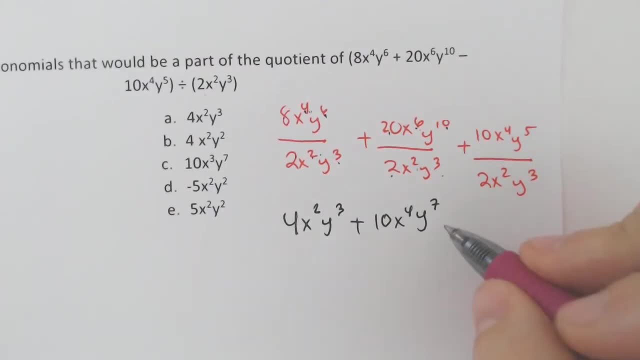 10 take away three, you get Y to the seventh. 10 divided by two is five. Oh, it was a negative 10.. Negative 10 divided by two is negative five. Four: take away two, you get X to the second. 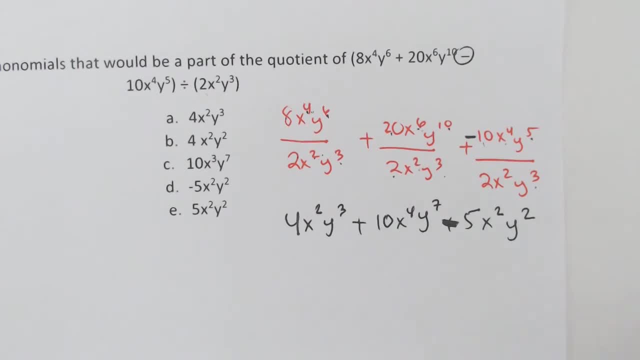 Five. take away two, you get Y to the second. All right, so let's see which one of these answer choices are actually here. Four X squared Y to the second, All right, so let's see which one of these. y to the third, a 10x to the fourth. y to the seventh- Oh nope, they didn't include it. And 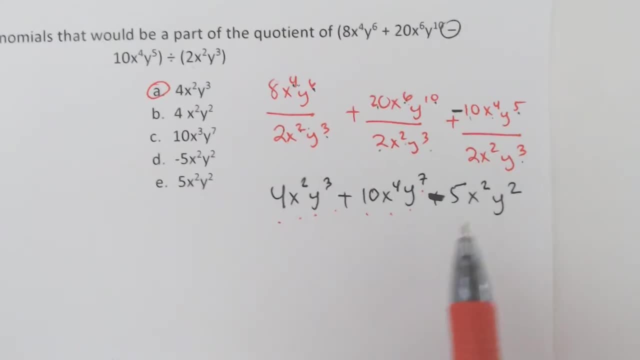 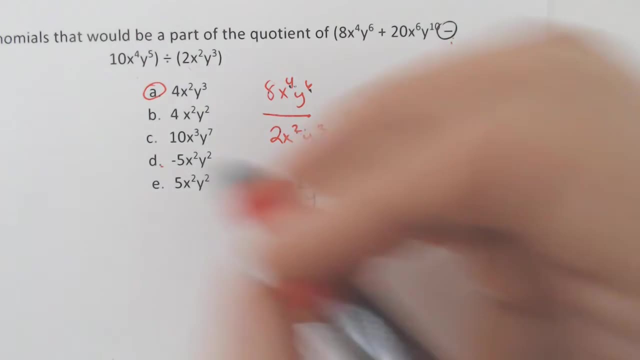 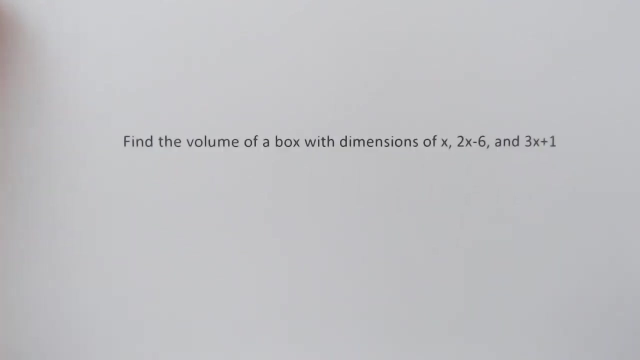 that's okay. You're selecting all that would be there, but it doesn't necessarily have to include all of them. Negative five: I almost missed that. negative Negative five: x squared y squared d. Okay, Keeping the trend alive, continuing and getting this video done for you. So we got. 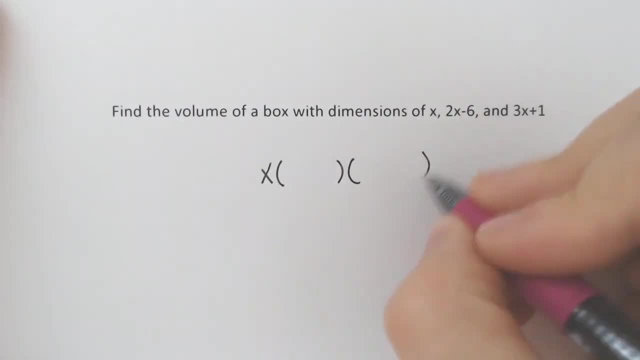 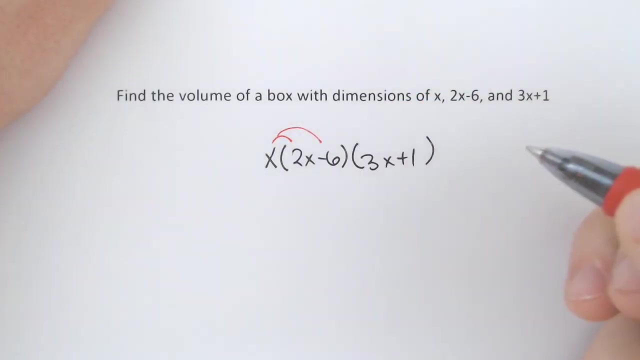 find the volume of a box with these three dimensions. If you want to find volume, volume is just length times width times height. So you can do length times width times height And I would recommend distributing the x first. perhaps Get it out of the way, That would be 2x. 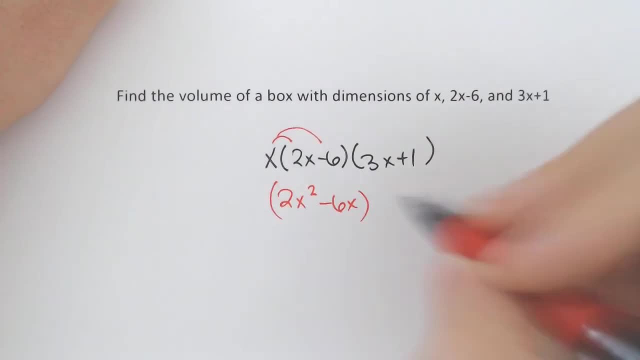 squared minus 6x times a 3x plus 1, which you would then just foil as well, like normal. So 2x squared times 3x is 6x to the third, because you add your exponents, 2x squared times 1 would be. 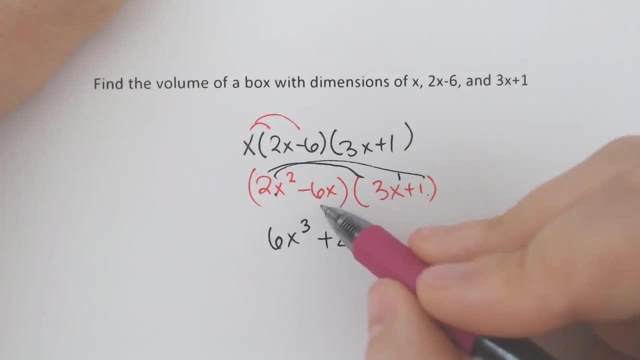 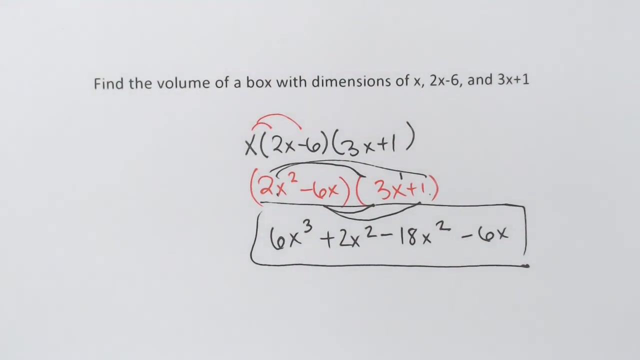 2x squared, Then negative 6x times 3x is negative 18x squared And negative 6x times 1 is negative 6x. And that, ladies and gentlemen, is that problem. All you had to do was foil it. 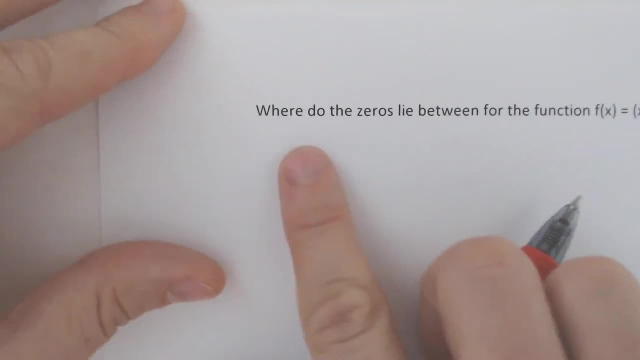 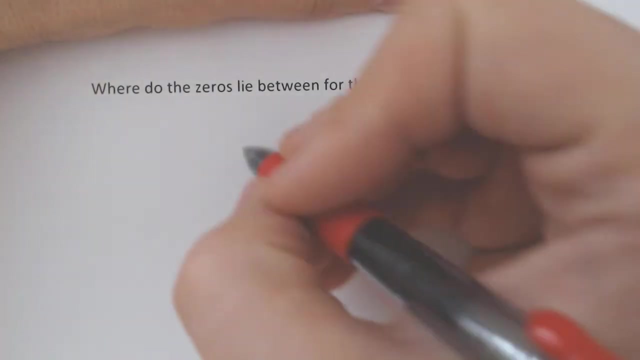 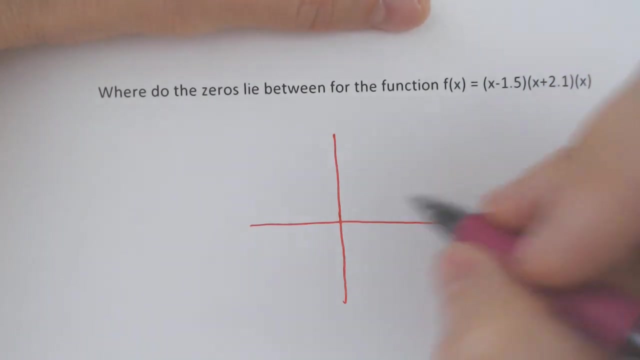 Next one, This one right here: Where do the zeros lie between for the function? So, where do the zeros lie between for this function? You have the choice of graphing it in your graphing calculator, but you also have the choice of using your noggin, your brain, and knowing that if it's x minus 1.5,. 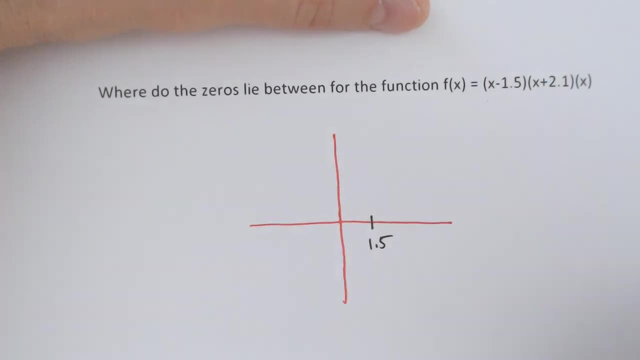 you could change the sign to get 1.5.. You could change the sign to get negative 2.1.. And then, if it's just x, that's 0.5.. 0.. Okay, so that's the weird one, And if you did graph it it would look kind of something. 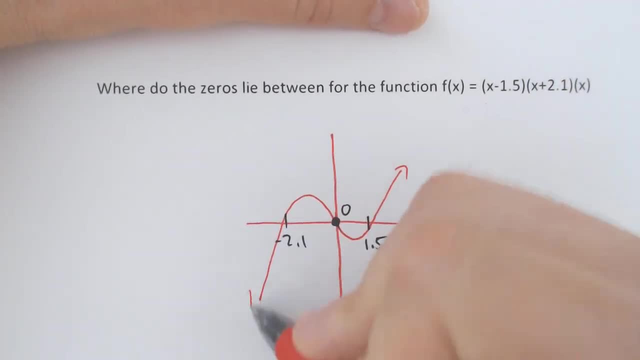 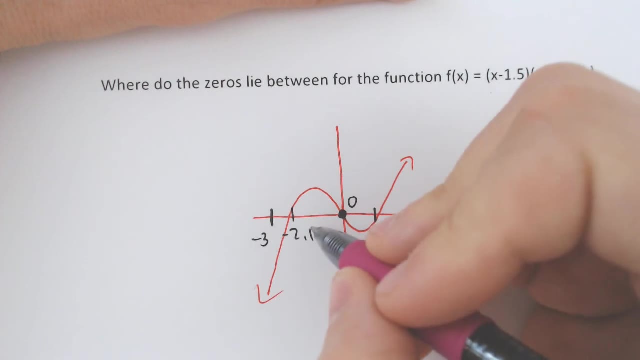 like this. Not that it matters, because the question is asking: where do the zeros lie between? Well, it lies between negative 3 and negative 2, because that would be where negative 2.1 is. So that would be one of the answers: negative 3 and negative 2.. 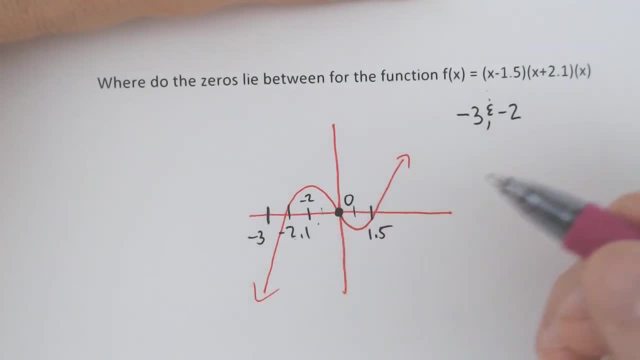 It also lies between, I guess, negative 1 and 1 for the 0 one, but like- oh, I don't know- negative 1 and 1 for the 0, but it goes through 0. That one is a no-brainer, So that's your 0.. 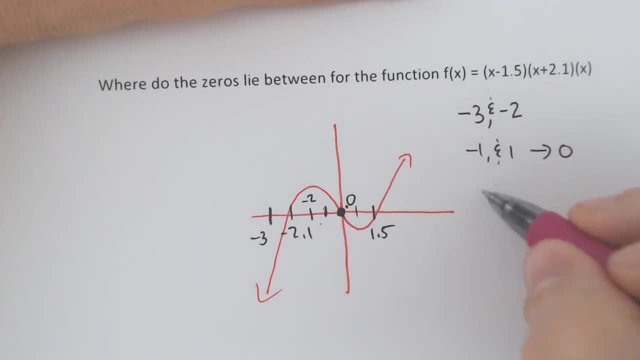 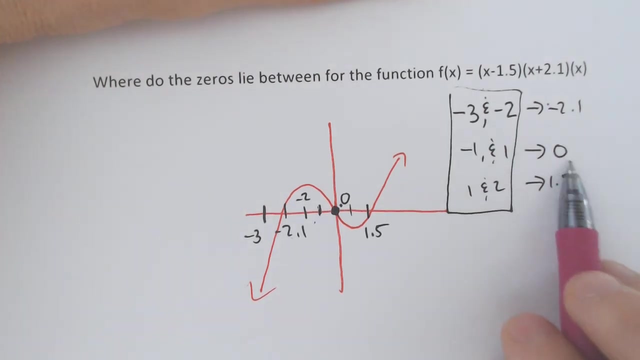 And then it goes between for the 1.5.. Well, 1.5 is in between 1 and 2.. Okay, So your three answers that you should really have would be these right here, and they relate to the 2.1, the 0, and the 1.5, respectively: